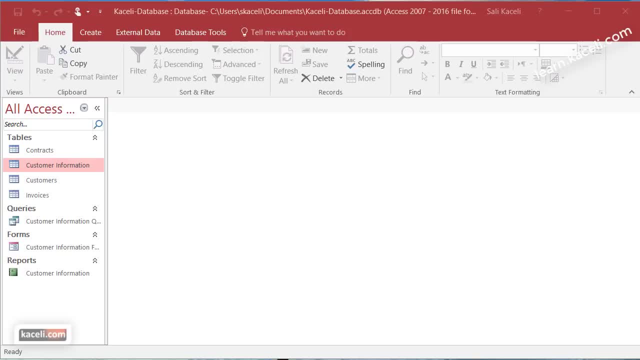 And typically the key component for linking tables in a database is the proper design of the tables to start with, And typically what you want to do is that you want to have the primary keys and the foreign keys properly defined in the tables. Before I further explain this, I'm going to clean up our database. 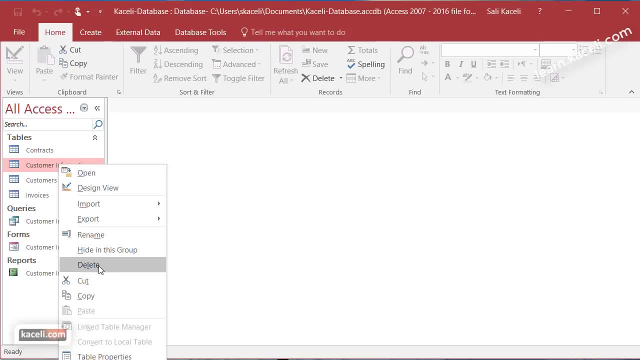 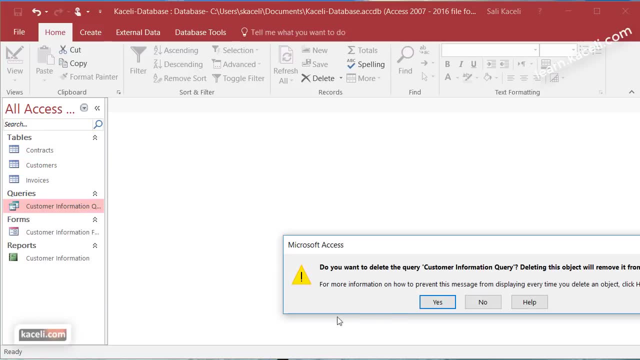 So I'm going to first delete this table. that has nothing to do with what we are planning to do in the next couple of minutes here. I'm going to delete these queries as well. By the way, you don't want to do this on a real database, unless you're sure that you want to delete this. 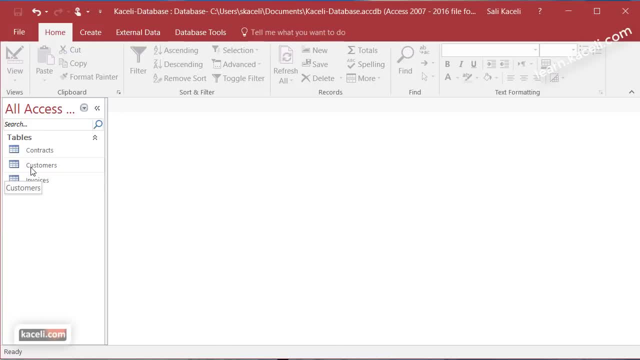 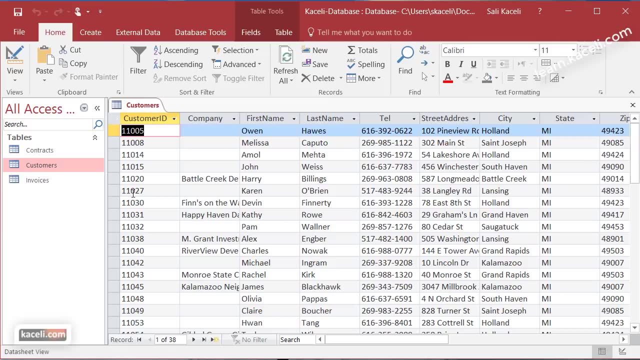 And at this point we have three tables. So we have the customers table, we have the invoices table and the contracts table. To learn how we did this, please refer to the previous tutorial. We have the primary key For customer ID. this is the primary key for this table. 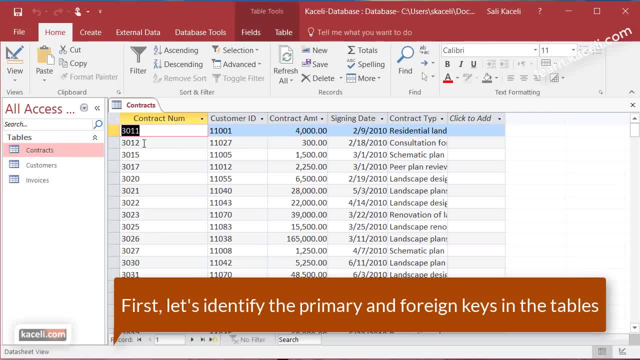 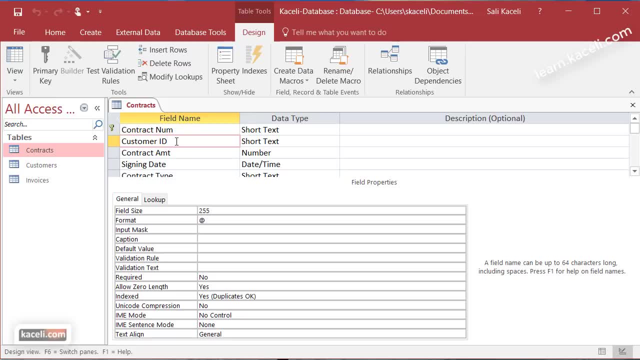 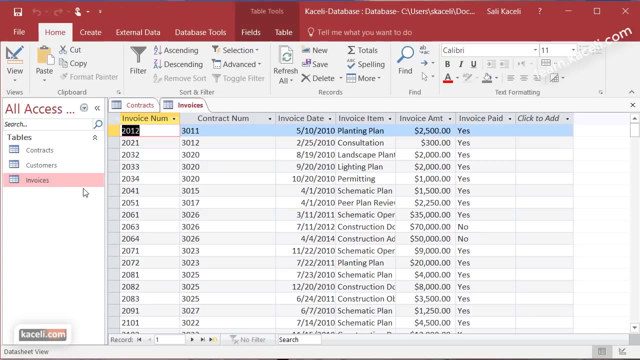 And then, under contracts, we have the primary key being the contract number, And then the foreign key is the customer ID, which is supposed to match with the customer ID, which is the primary key on the customers table. And then, the same way, under invoices, we have the invoice number, which is the primary key for the invoices table. 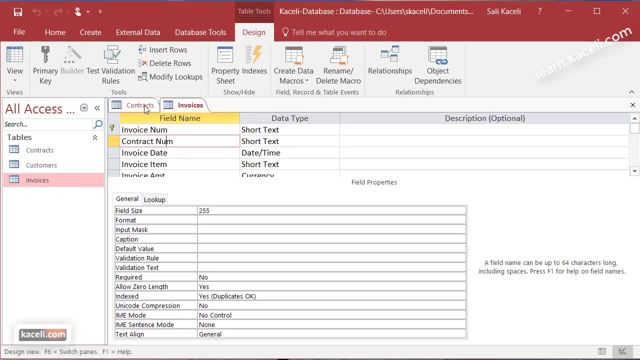 contract number, which is the foreign key in this case, goes to match with the primary key of the contracts table. So, as a design that the database you need to factor in and plan on what the foreign keys are going to be and how the tables are going to be linking with one another when it comes time, 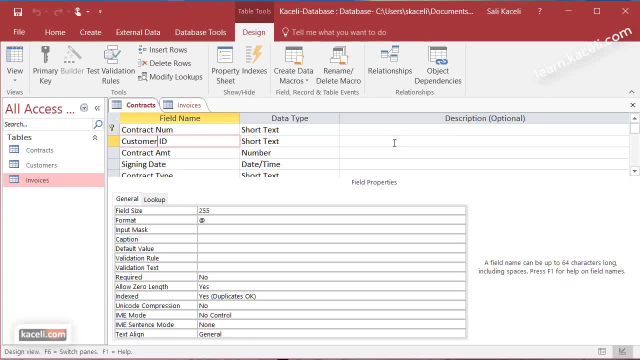 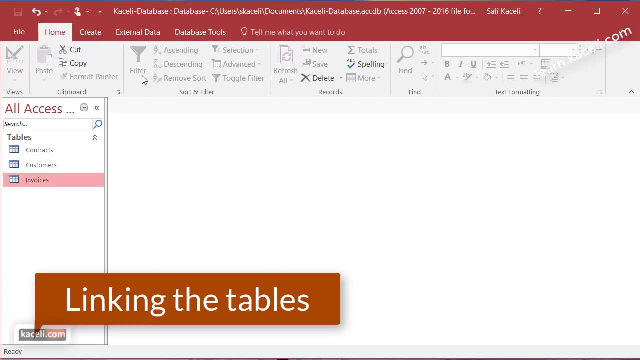 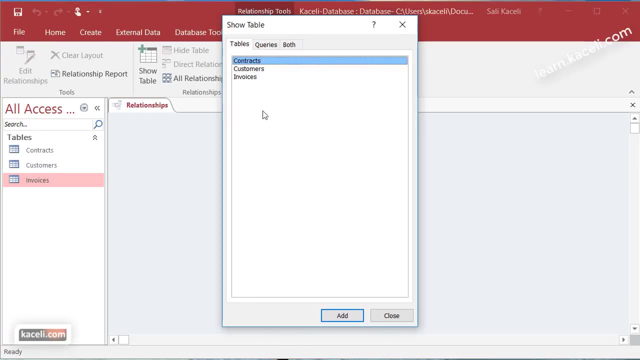 to link them, and this has to be done during the design process. Now, at this stage, we need to close the tables, and then the next thing that we need to do here is we need to go here under table tools and then we're going to define the relationships. So we go here under relations and then we choose. 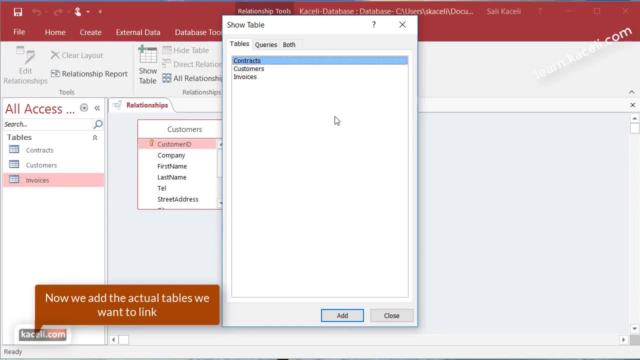 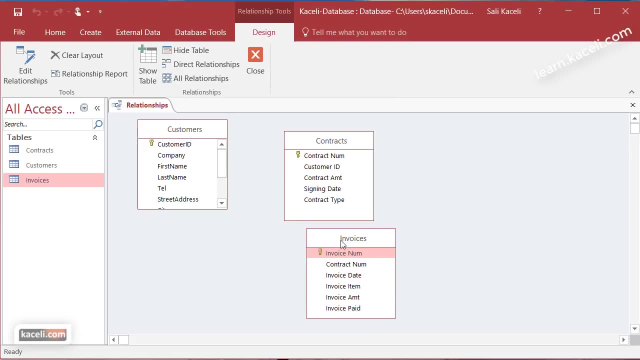 to add the customers table. We choose to add the contracts table and then the invoices table and then close this. Now notice: you can even organize them any way you want here. You want to organize them fairly logically, if you can, so that you see the structure depending on how you organized your. 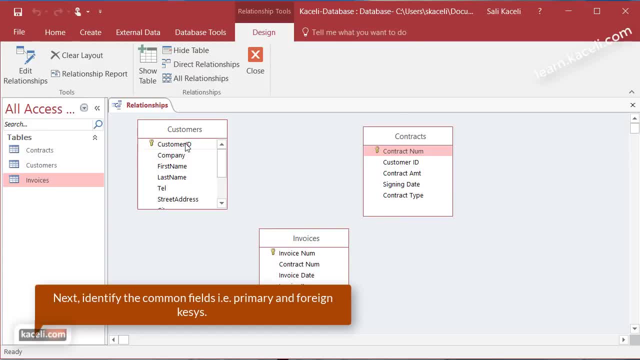 database To link those tables together. notice, we have here customer ID from the customers table and we have the foreign key here under contracts for the contracts table. So what you do is you click on customer ID from the main table and you drag it and you hold the mouse directly on customer. 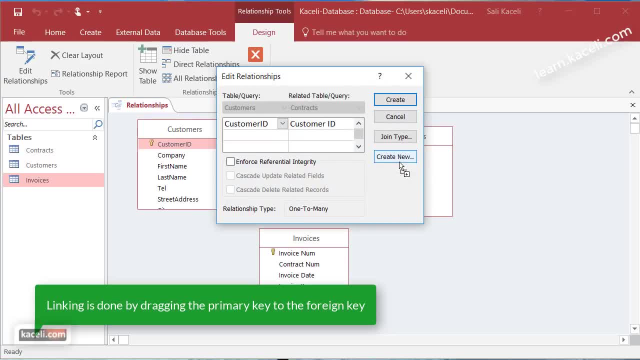 ID on the contracts table here and then you link the tables together. So you can see that the relationship between customer ID and the contracts table is going to be one to many. Now at this point. notice it's saying it's going to use the customers table linking to customer ID in the contracts table. 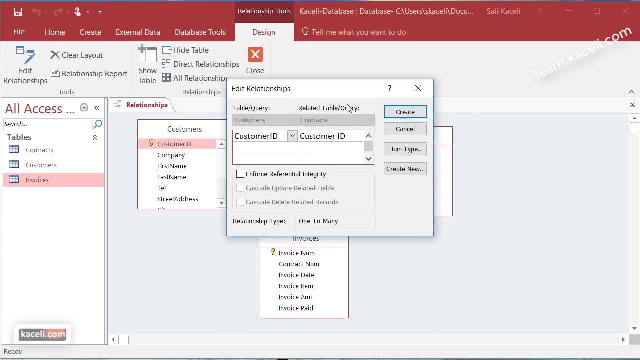 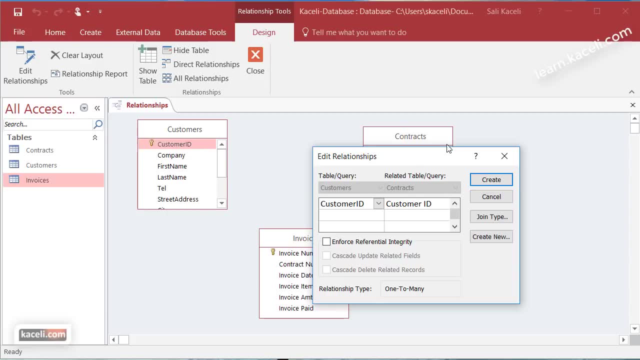 It's going to be a relationship of one to many. What that means is that you can have one customer with multiple contracts, and that's hopefully what you want. If you have a small business, you want multiple contracts from the same customer. You could also enable here what's called the referential. 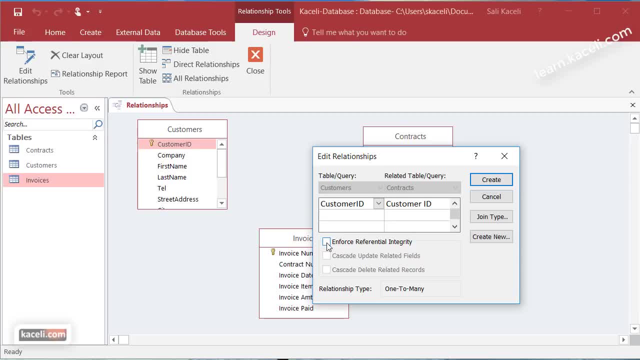 integrity. I'm not going to check it for now to keep this simple. but that means that if you deleted a customer, you're probably never going to have that customer again, then you want to delete also their contracts. That's what their referential integrity is. It's going to do a cascade update and cascade delete If you remove the main source. 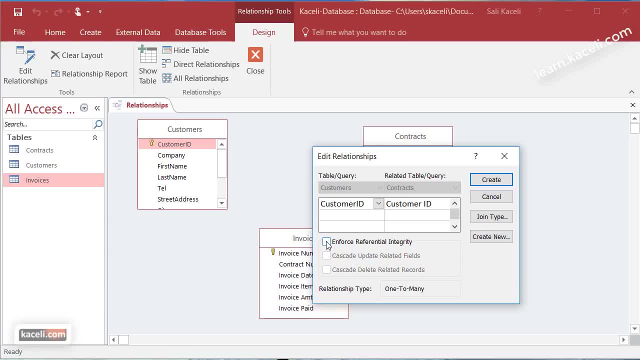 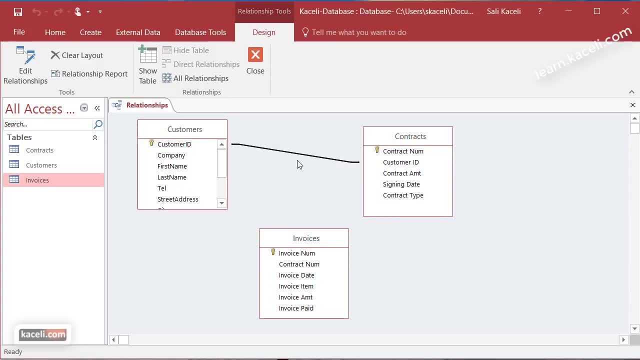 it's going to remove the items that follow with it. If a student drops from college, you want to drop also the courses and things of that nature. Then here we click on create and notice that you have a line between the two. The next thing that you want to do then is notice: now we have. 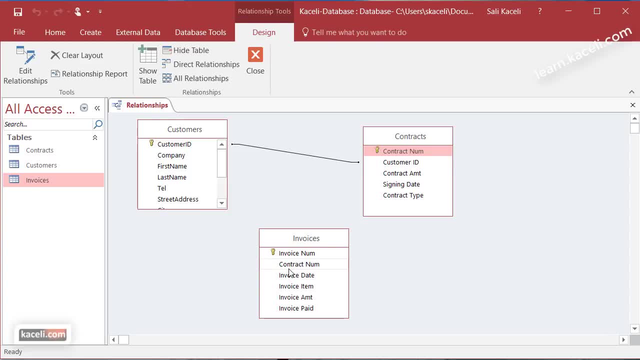 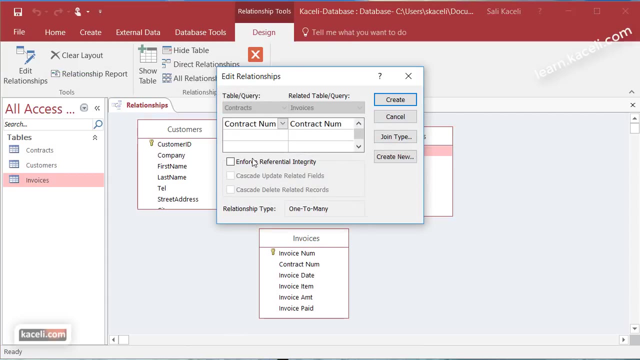 the contracts primary key here could link with the foreign key from the invoices table. So we want to say from invoices here we want to drag this to the foreign key from the invoices table. Again the same idea: contract number to contract number, one to many relationships. that means that you 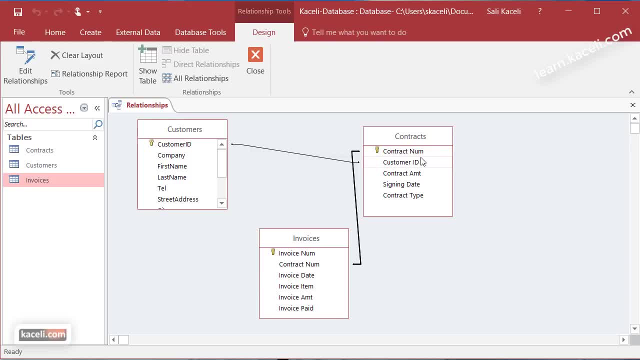 have multiple invoices for the same contract. That's what that means And, by the way, you can move this however it makes most sense to you. If, for some reason, you chose the wrong thing, notice that they have to match here. customer ID has to be under customer ID. it can be linked to a. 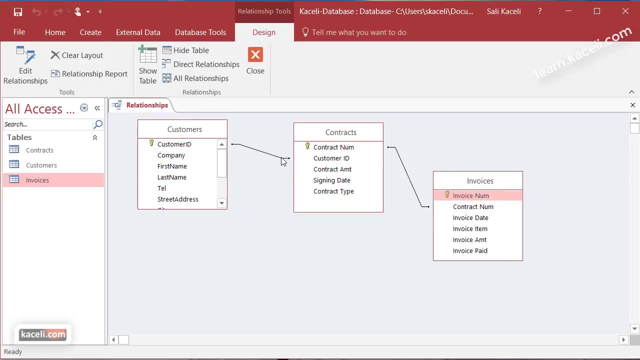 different field. If for some reason you had it improperly matched there, you can right-click so or select it once, and then you can choose either edit relationship or simply delete, And then, if you want to delete it, you say yes, and then now it's disconnected And then you can redo. 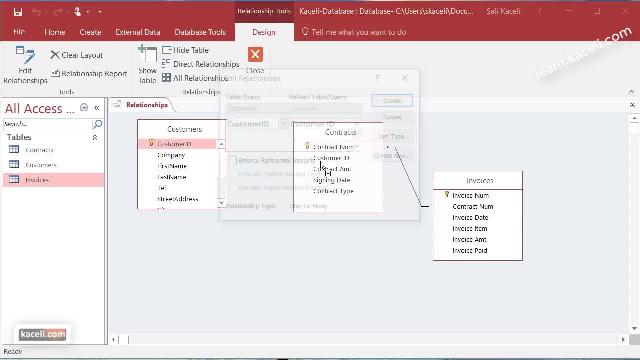 it again. so you just drag here customer ID to customer ID and then click on create again, and now you'd have it the way you wanted it. Once you're all set with this, you need to click on close, and that's where the system is going to save these links between the tables, because unless the 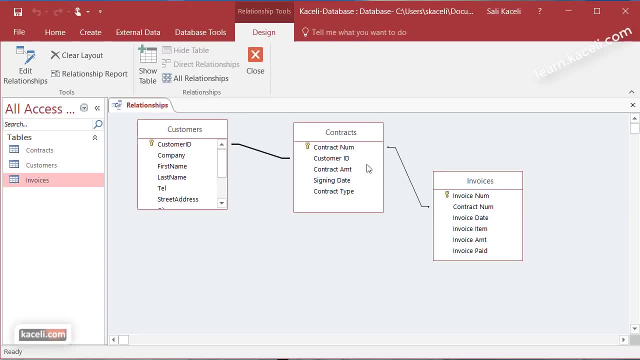 tables are linked together. we cannot get data from one table to the other, And when we link these tables through this relationship that we can actually go and say: I want, for example, a query here or a report of some sort, that I want the first name, last name, and then I want the contract. 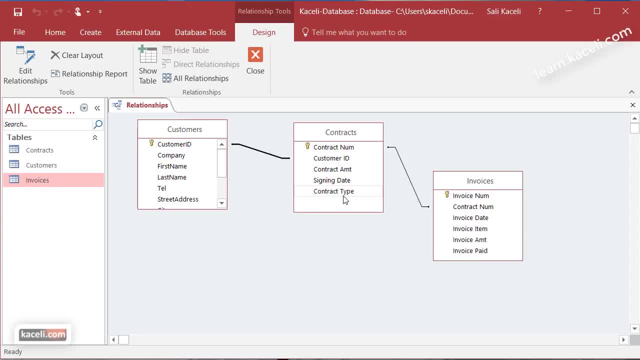 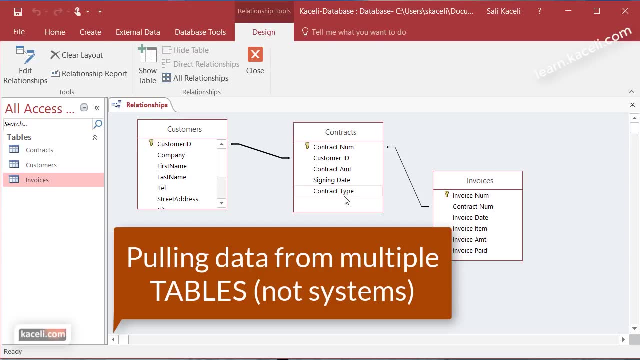 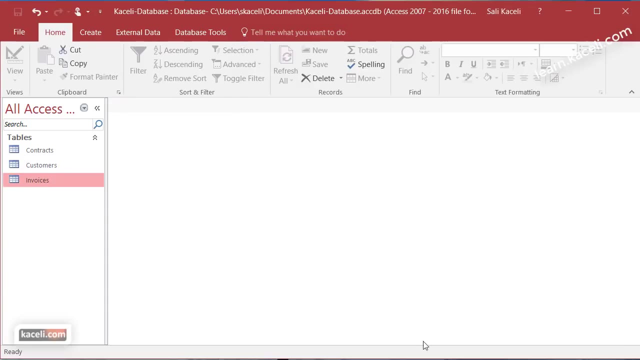 number and then I want the amount and the date and the contract type. That's when you can kind of cross and pull the data from multiple systems. So if we click here on close and then it's going to ask us to save the relationship, here we say yes. 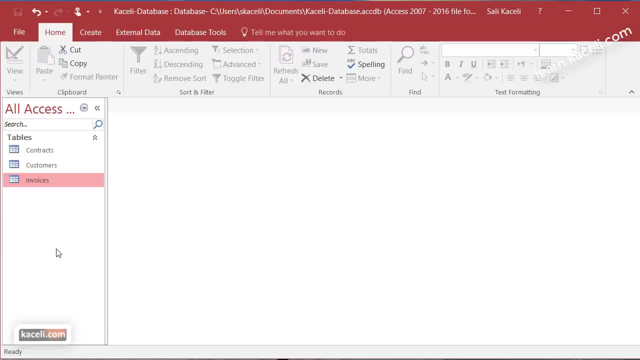 and now the relationship has been defined and now we can actually create queries, we can create reports, we can create forms to pull data from multiple tables here. So this is where the beauty of Microsoft Access actually takes place. Let's very briefly learn, just for the sake of testing, at: 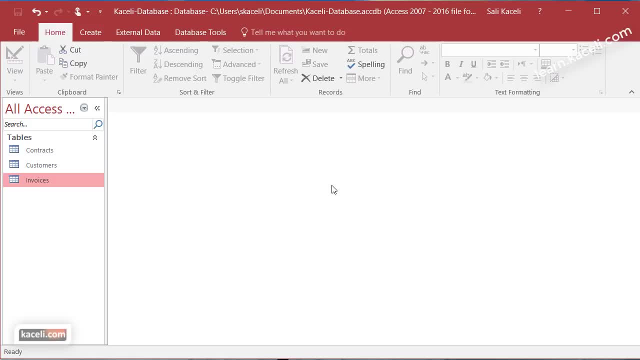 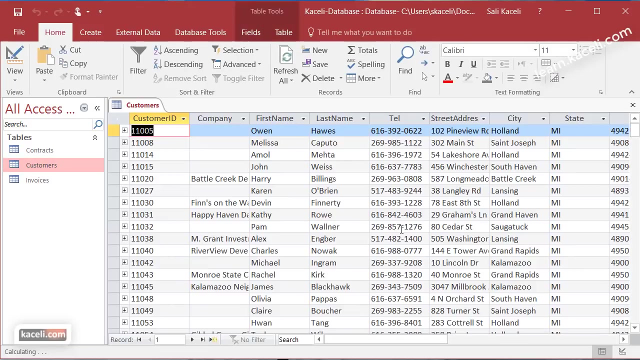 this point, how to create a quick query on pulling data from two or more tables just before I finish this section. so you get an understanding of how the relationship connection here between the tables, what the advantage is. So if we were to look here at customers notice, I have the customers table but I 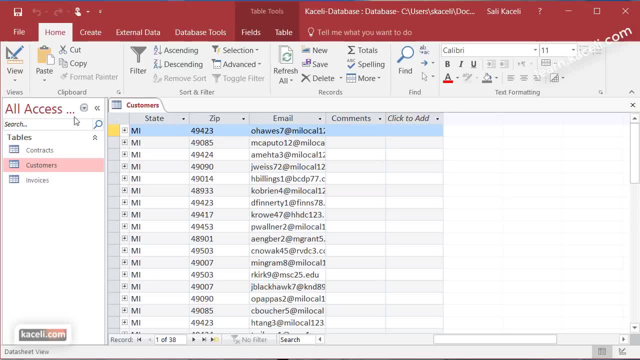 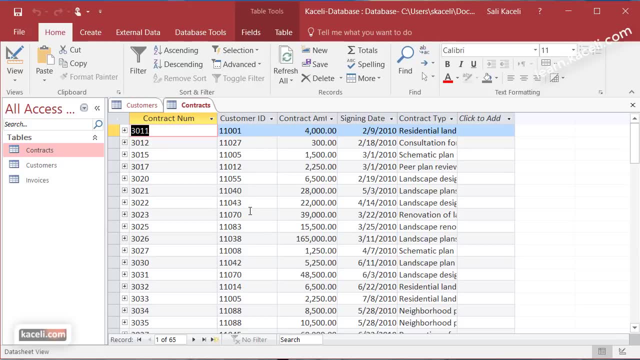 don't really have any contract information for this customers table And if I go to contracts I have only contract information, but I don't really have any customer information other than this ID. So now that we've done that we want to do is we want to pull the customer information and the contract information and have it. 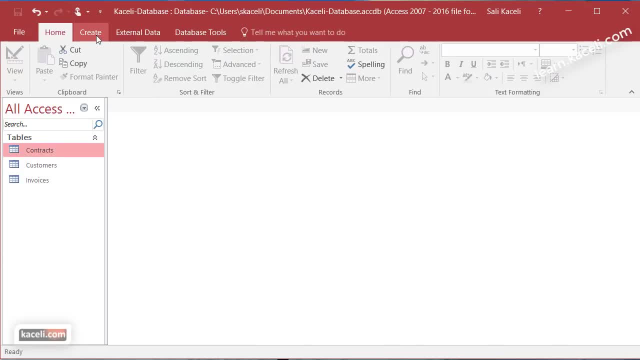 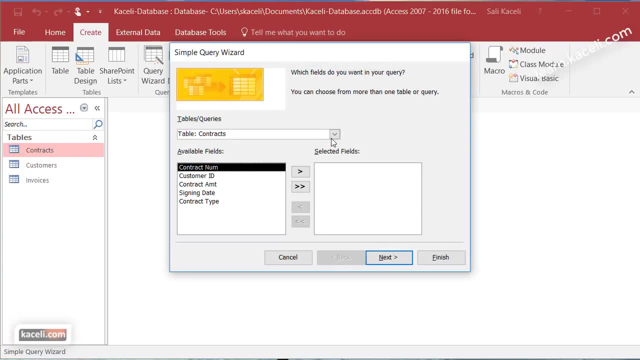 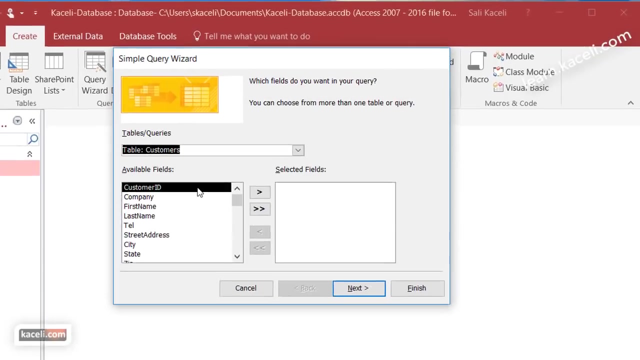 displayed a certain way. So here's how it works: You go here under create and then you go under query wizard and then we click on OK And then we want to pull here first from the table. customers Notice that we have three choices where we can choose from. So we choose customers and then now it's. 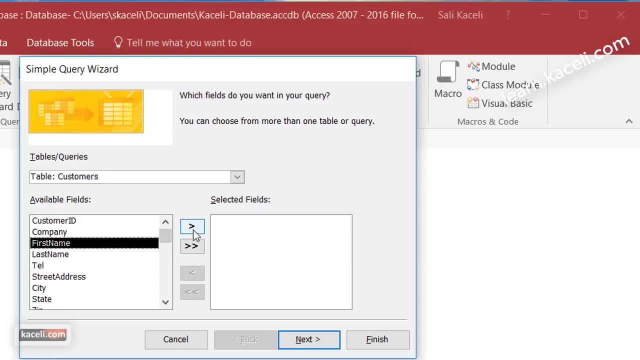 just a matter of whatever we want here. So we say I want the first name, The last name, And then let's say: I'm interested now from that table, I'm interested on only these two fields. The next thing that I want is I want to go under contracts and then I want to pull here the 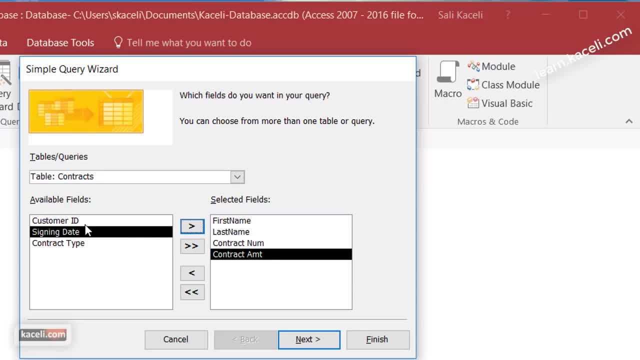 contract number. I want to pull the contract amount. I don't care for the customer ID because I know I have their first and last name already, And then I want to see the date and the type of the contract. So notice, it's about six fields here from two tables. Now I click on. 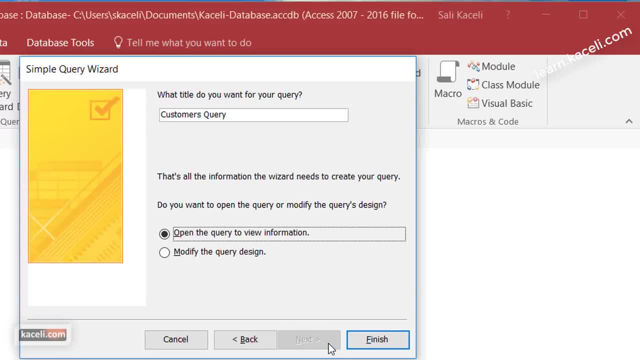 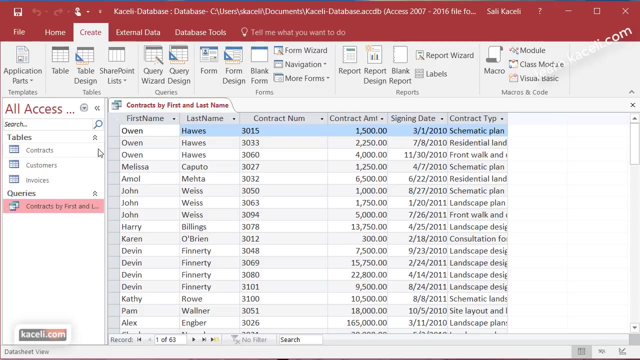 next and then click on next again and now give it a meaningful name. So whenever you're defining the queries, you want to define it with a meaningful name. Contracts by first and last name. Click on finish and now notice that we have a new query created and now we have the data: first name and 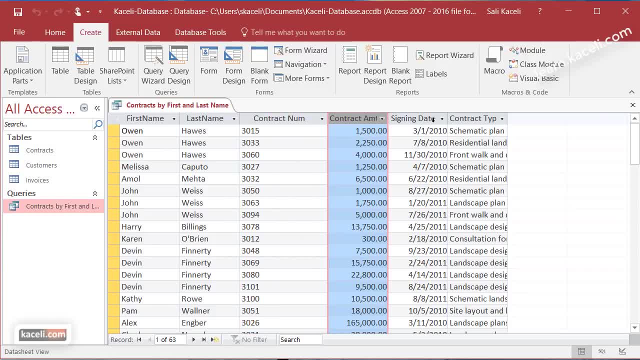 last name and a contract number and then the amounts, the date and the type. Notice, so we pulled the data from two tables. From here you can see the table and the date and the type. So now you can create all kinds of other things, whether it's reports or new queries or forms, and we'll 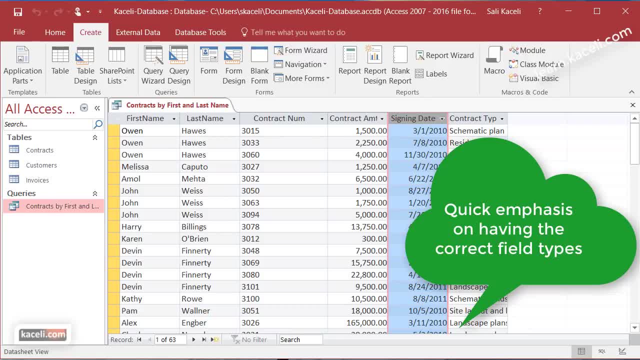 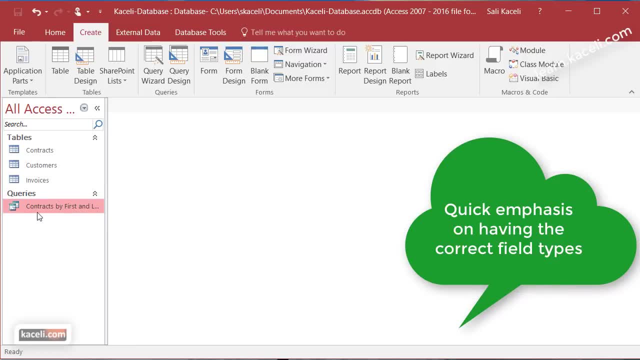 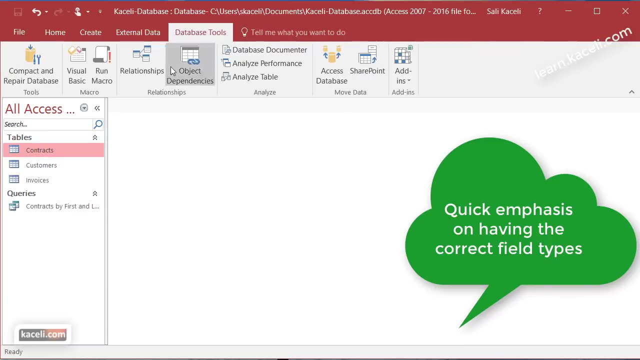 cover those in the next few sessions. One other thing before I finalize this session- and I should have mentioned it earlier- is is that in order for you to link those tables correctly, you need to make sure that the fields that are going to be linked through the relationship are of the same. 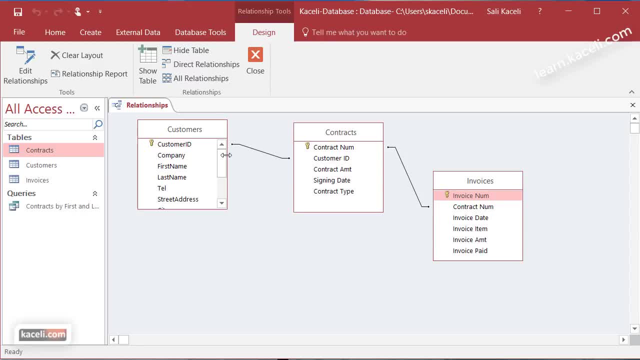 data type, And this is where a lot of users get frustrated because this does not work. What that means is is that on the customer's table, when you go to design your table, you need to make sure if that is a number field, if it's numbers, 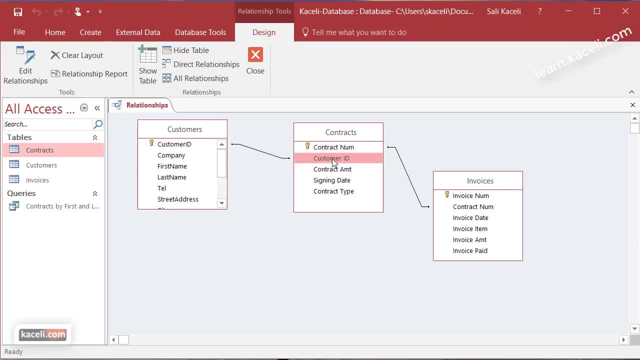 you need to make sure that this customer id over here. on the next table in the foreign key, it's actually a number field as well. It's the same type of field Again here, the contract number on this table, on the contracts table. that needs to match exactly the same as the number field.